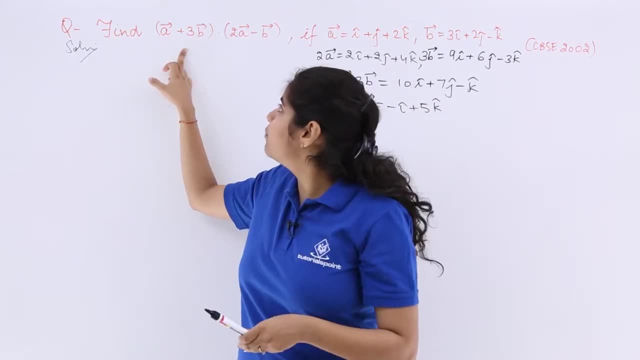 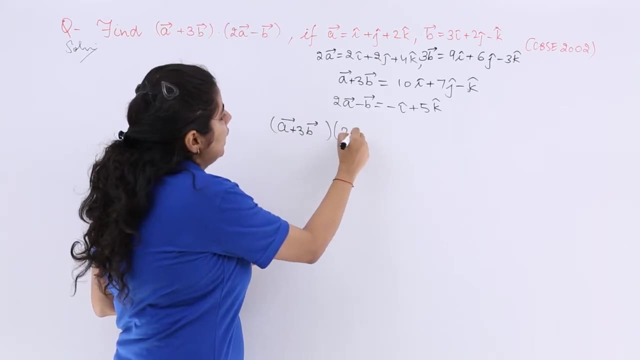 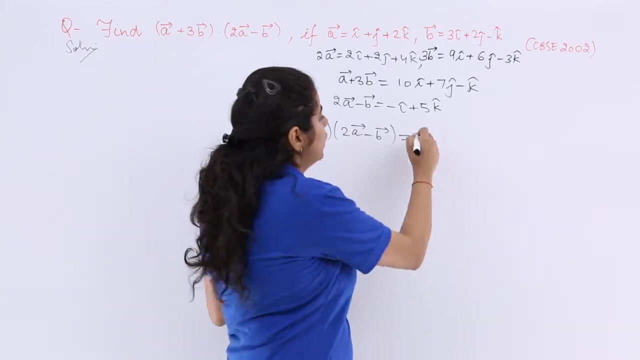 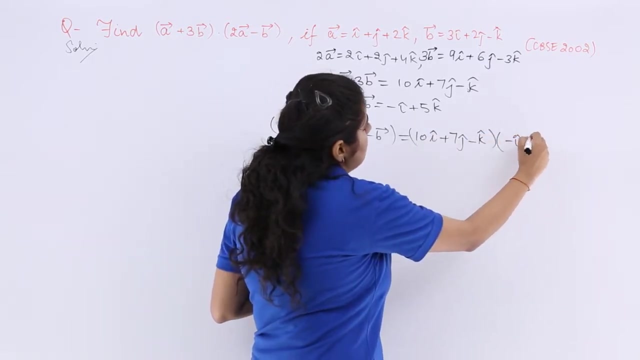 Now the dot product has to be formed from a plus 3b multiplied 2a minus 3b, So a plus 3b, So a plus 3b multiplied 2a minus b, not 2a minus 3b. Now what to do? You have to find the dot product of 10i cap plus 7j cap minus k cap, multiplied minus i cap plus 5k cap. 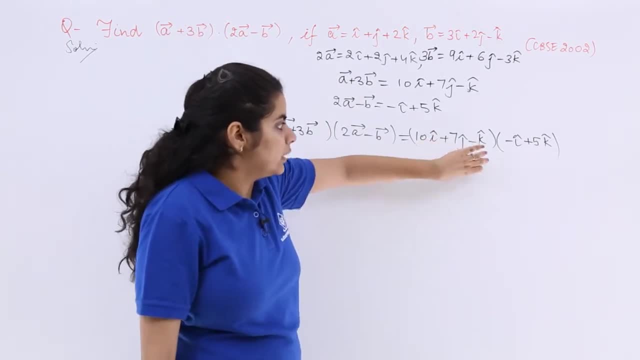 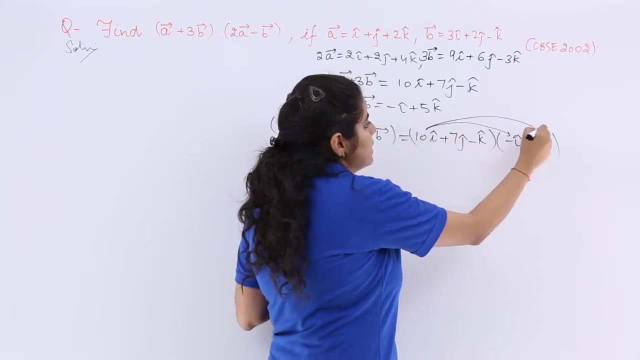 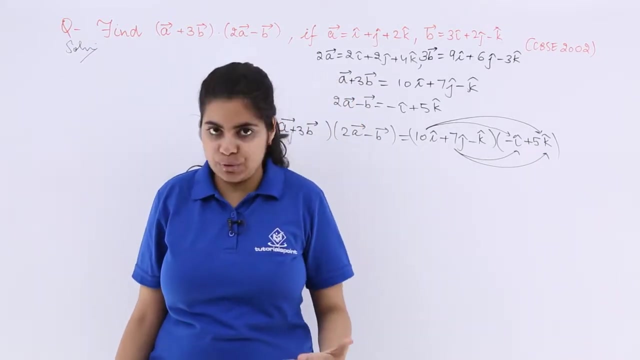 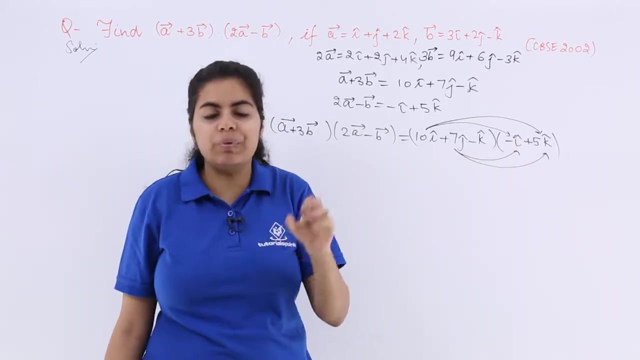 Now let's multiply. We know that. see, these are two terms being multiplied. So in mathematics, also in algebra, you use to multiply like this. Then these terms were multiplied and the last terms were multiplied. Right, But now what we have to do is- we have to make this very clear: that 10i multiplied by minus i can be done, because i cap, dot, i cap will be what. 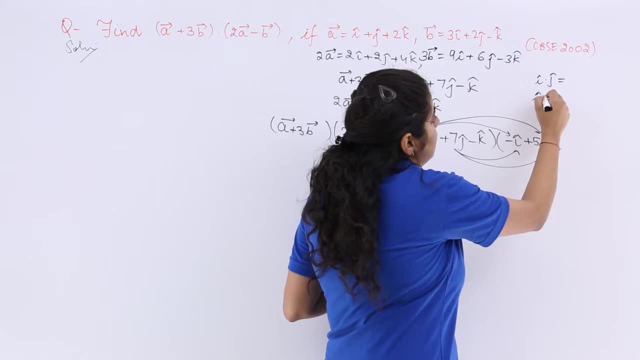 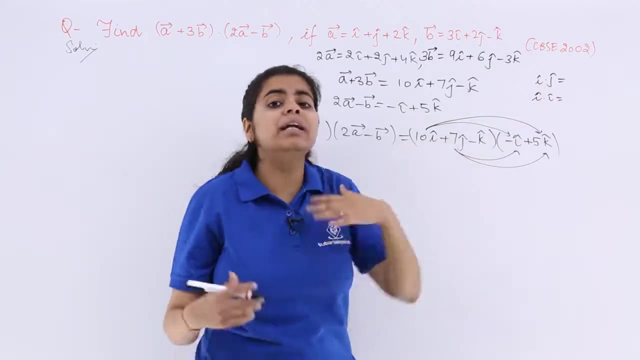 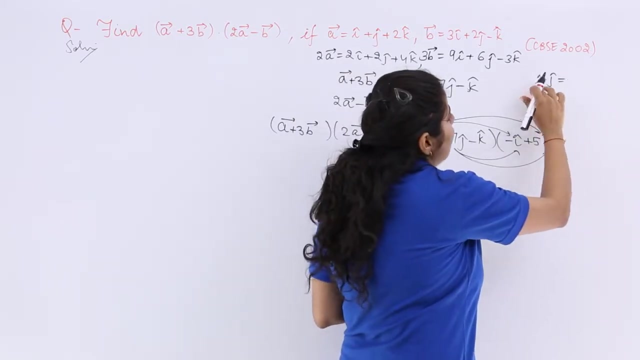 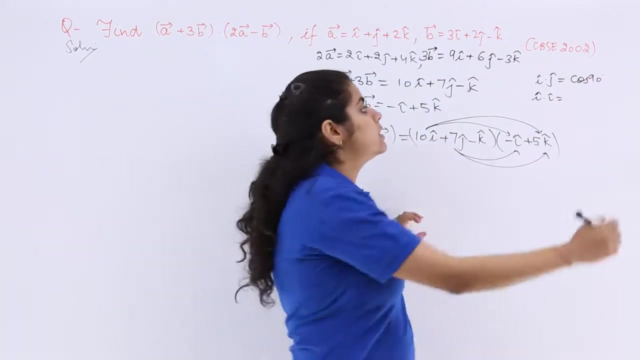 See: i cap dot, j cap and i cap dot. i cap means a unit vector when multiplied by itself, or a unit vector multiplied by different unit vector. What should be the answer? So this will be like: a dot b is equal to ab cos theta. So i j cos theta. What is theta? Because these are mutually perpendicular cos 19.. So it will be 0. 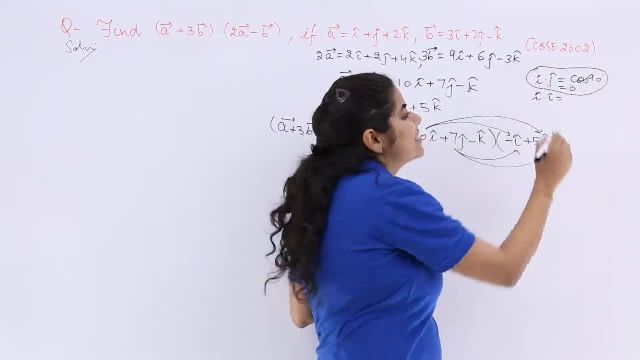 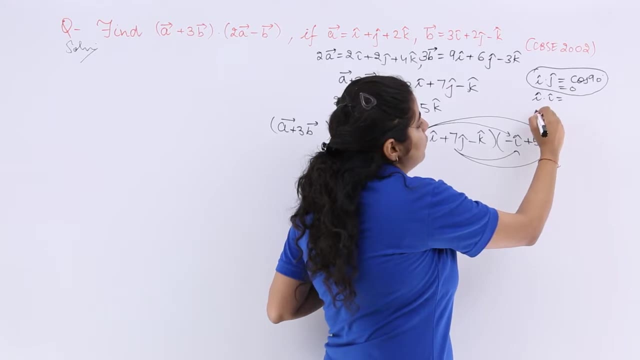 Means. any two unit vectors which are not same and they are in the scale of product, will yield me 0. But here you see, it is i into i, which is 1 cos theta Between i cap and i cap. what is the angle? 0 degree Right. 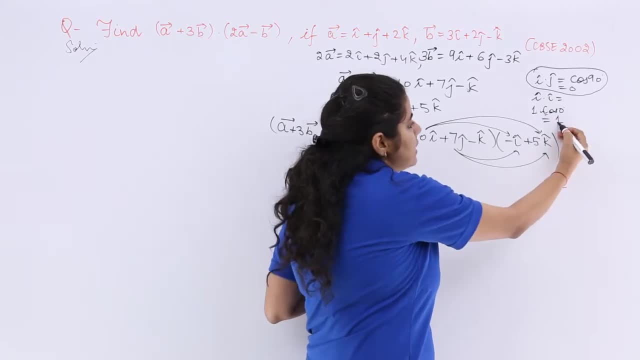 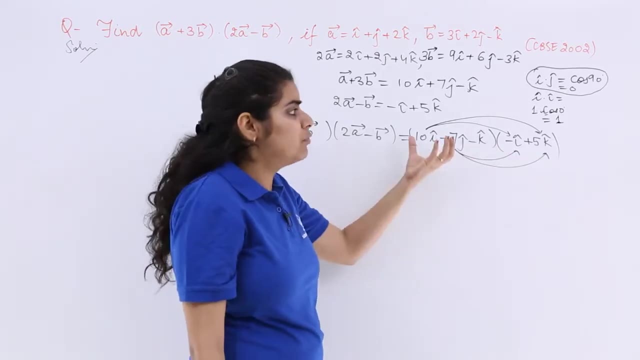 So 1 multiplied by cos 0 is 1.. Hence the answer is 1, here and there it is 0. So that means wherever you have to multiply, you have to take only those terms into account which actually are unit products multiplied by each other. So 10i multiplied by i is 10 into 1 is 10, but minus sign should be there. Then this 10i when goes with 5k, this will not be considered, because i cap, dot, i cap will be 1.. 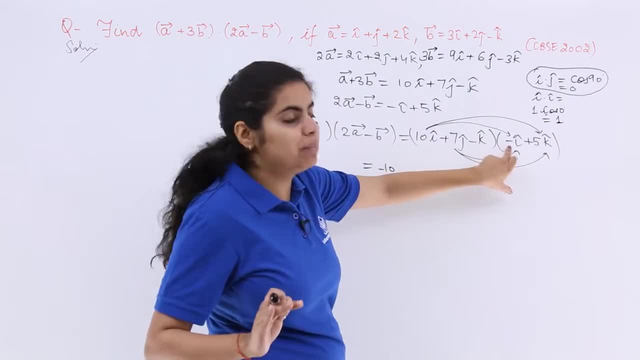 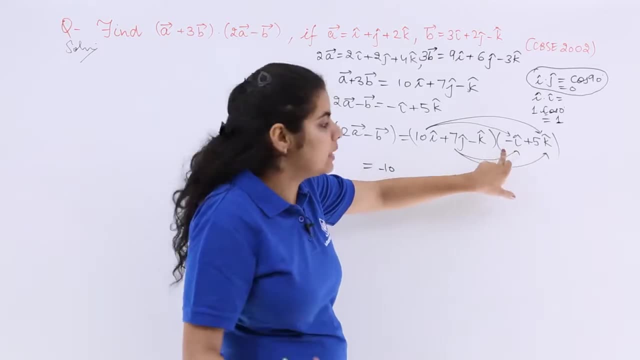 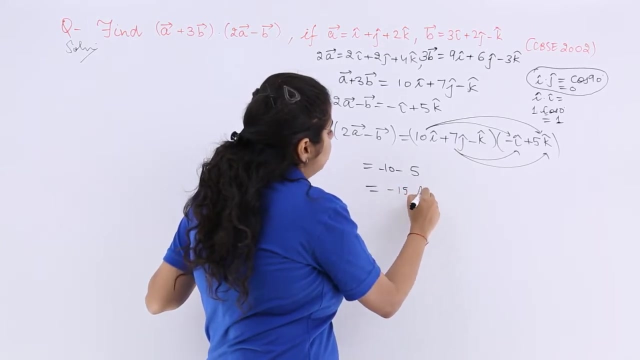 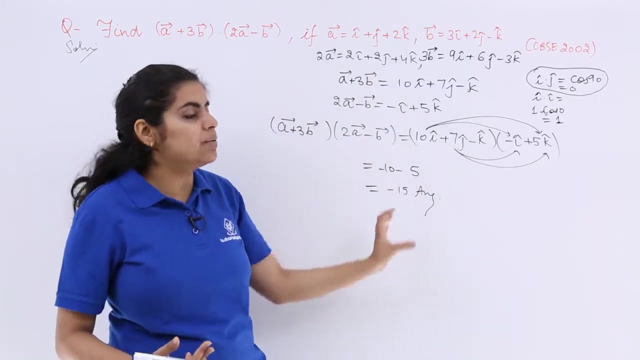 i dot k will also give me 0.. Then 7j multiplied by minus, i will not be considered. 7j with 5k will not be considered. Minus k with minus i will not be considered. Minus k with 5k will give me minus 5.. So this is minus 15. that is the answer to the dot product. So we have to make very sure that. what do we have to consider? This question seems very long, very typical, but in fact it is not. It is the basic of the dot product. Thank you.